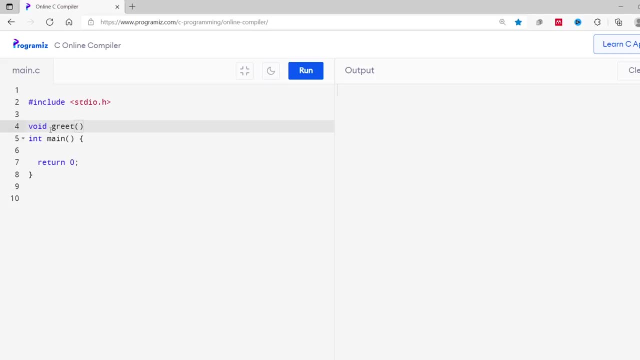 the name of my function and don't forget to use the parenthesis. These are needed to denote that this is a function. Now, inside the function, I'll print good morning. So good morning. Now let me run this code. As you can see, nothing happened. This is because to run a function, we need to call it Now. to call a function. 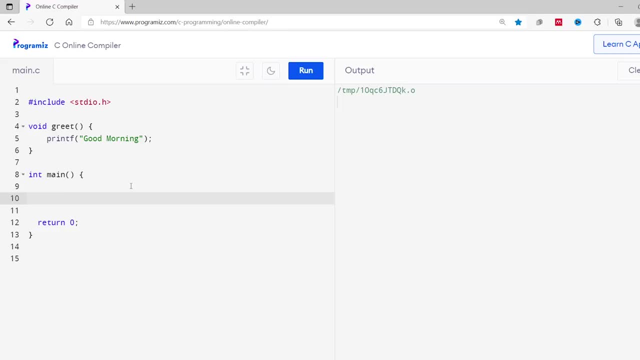 we use function name with the parenthesis. So we use the name of the function that is greet with the parenthesis, and i'll run this code now. this time you see the output. good morning, let's see how this program works. like any other c program, the execution starts from main, and when it encounters the 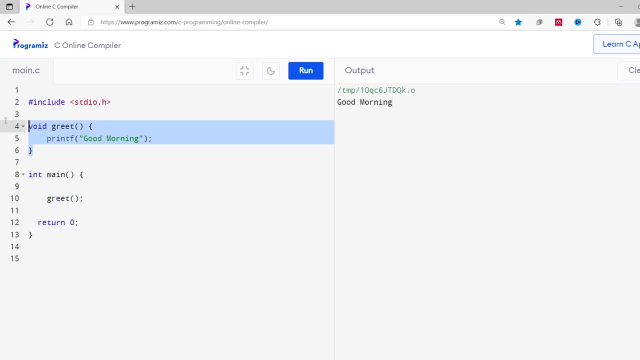 function call. the control of the program moves to the function definition. now the code inside the function is executed and good morning is printed on the screen. once the execution of function is completed, the program of the control moves back to the next line after the function call. now, to verify this, we can print the statement after the function call. so i'll print after. 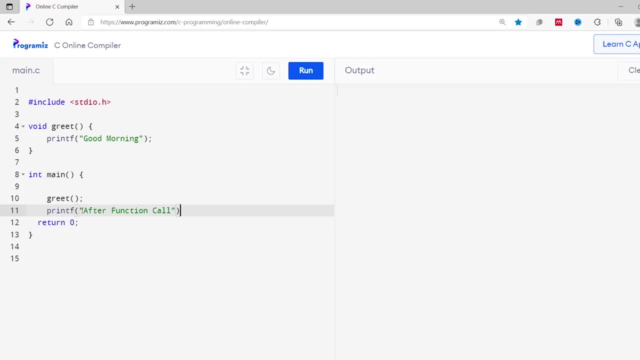 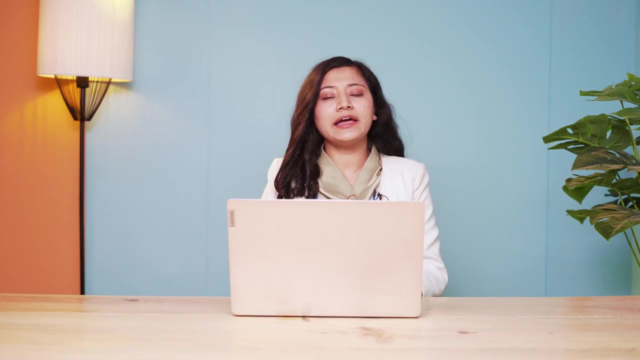 function call, and before i run this i'll add here backspace n. now let's run this, as you can see. first the code inside the function is executed, now the control move back to the function calls, so the code after the function call is executed, so we get the output. good morning. and after function call, and as discussed earlier, one. 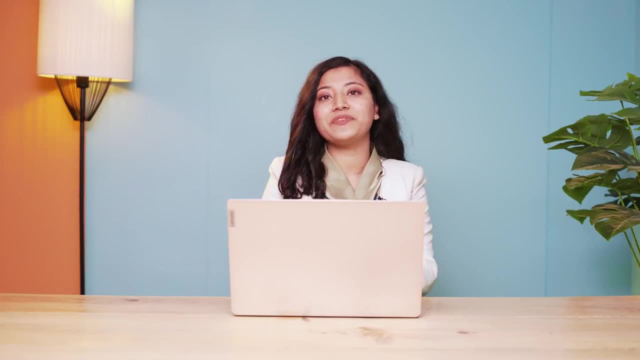 of the good thing about the function is code reusability. now, once we create a function, we can reuse it any number of times. all we need to do is call it whenever we need. now let me show you. i'll remove this print statement and i'll add: 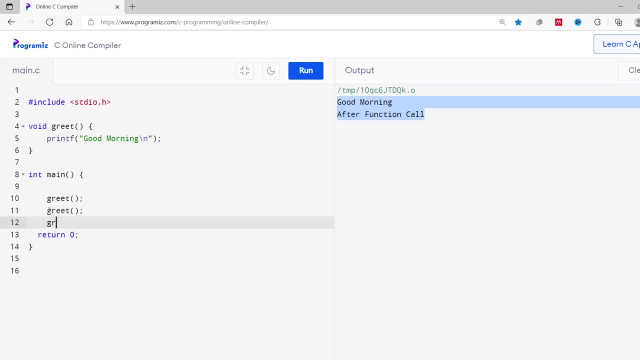 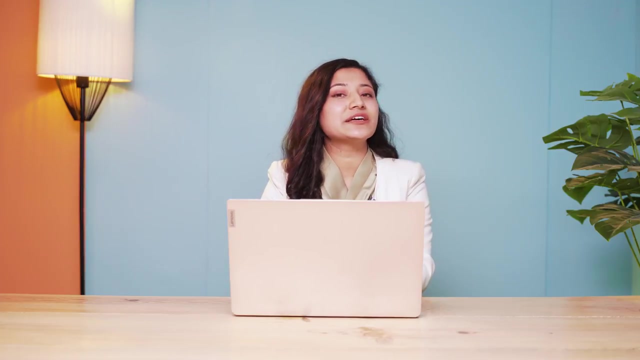 greet two more times. so greet and i'll run this. so this time you can see good morning is printed three times. before we move to the next section, here is a quick tip for you. it is a good practice to use descriptive names for functions so that anyone reading the code will know what the 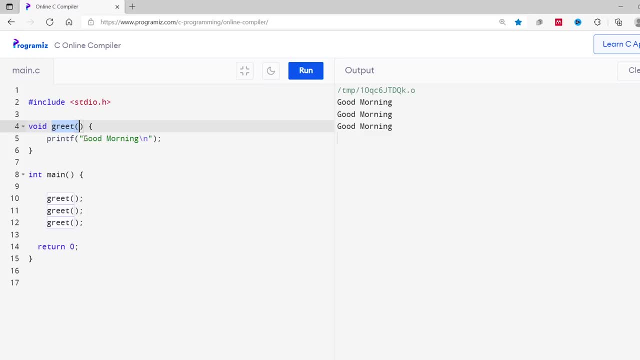 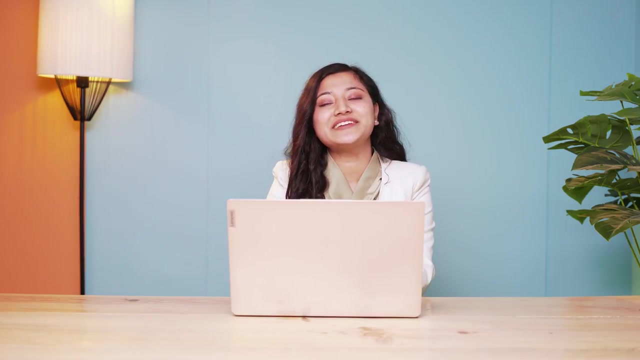 function is doing by just reading the function name. here we are greeting good morning, so we are using grit as its function name. we can also use wish morning or any other descriptive function name. by the way, if you are watching this, there is a good chance you want to improve your skills in. 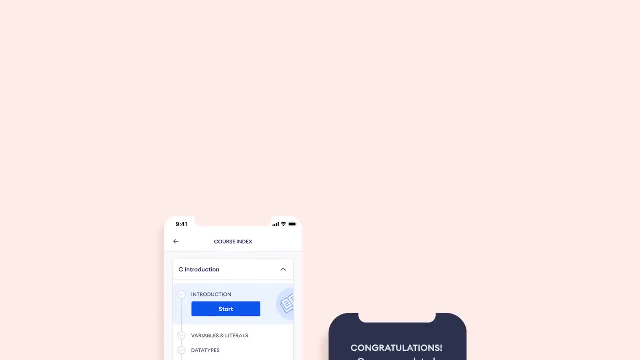 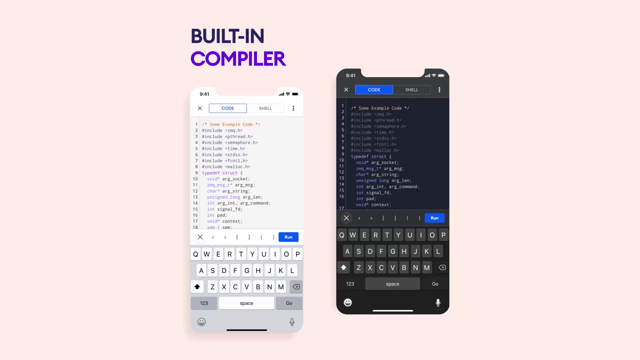 c programming. lucky for you, we have a mobile app that provides a well-structured c programming course with certification at the end, and you can use the app, alongside the video, to practice on the built-in compiler. our course is free, so download now by scanning this qr code or click. 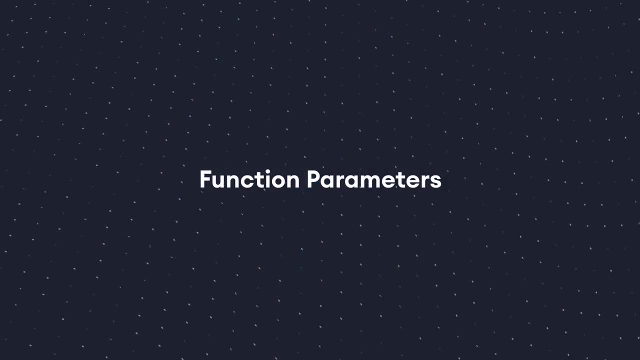 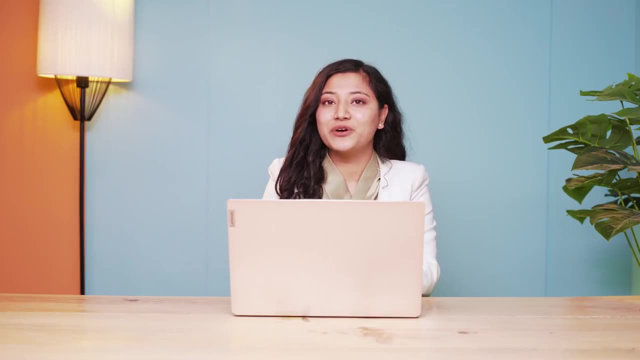 the link in the video description. so far we have created function that just prints message. however, sometimes we might want to create function that accepts some value and perform some action based on that value. for example, suppose we want to create a function that accepts a number and computes the square of the number and print it. we can do this in c programming with the help. 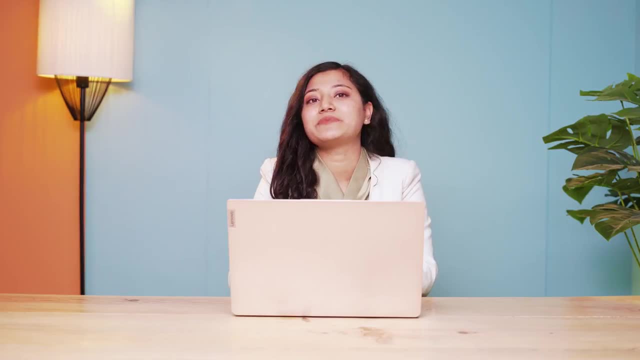 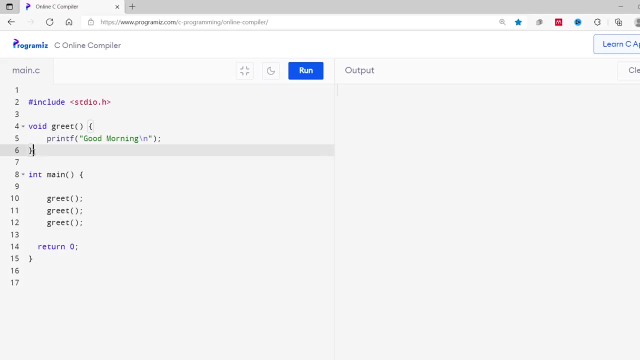 of function parameters. a parameter is a value accepted by the function. now let me show you how we can create function with a parameter. so let me get back to my previous code. i'll remove this grid function and i'll also remove this function call. now i'll add another. 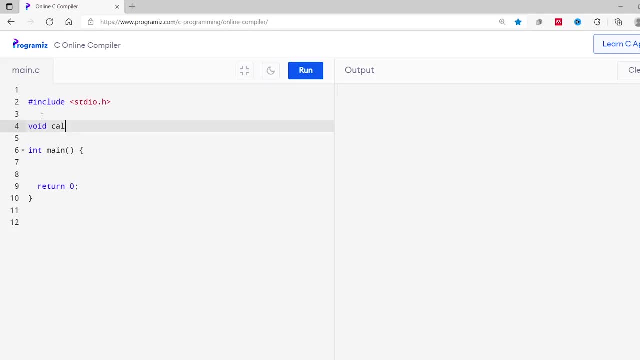 function. call it calculate square. so calculate square. and inside parenthesis i'll add function parameter: int number. now, inside the function i'll do: int square is equals to number multiplied by number. then i'll print the number and it's square like print f bracket inside quotation. square of percent d is percent d, that is after. 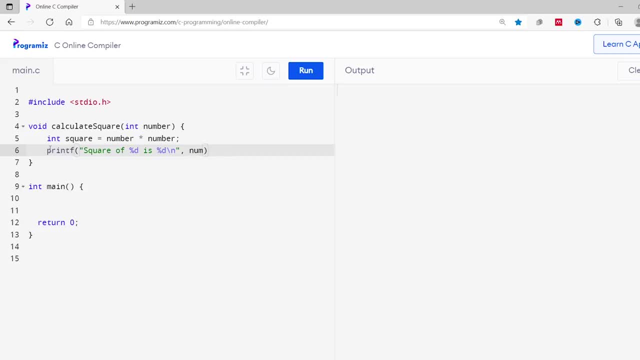 comma number- sorry, number, comma square. now here in the main function, i'll call the function: calculate square. now let me run this code. here we get an error. this is because when we create a function with a parameter, we need to pass the value while calling the function. so in the function call. 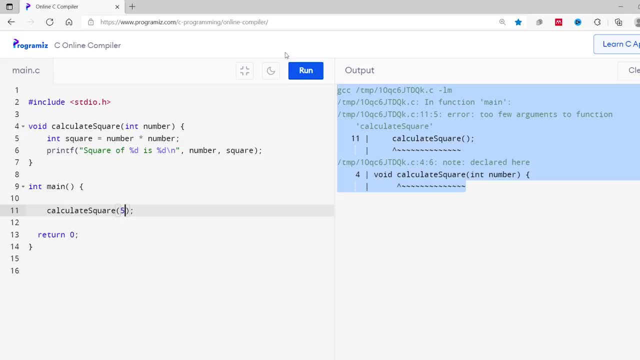 i'll add 5 inside the parenthesis. now i'll run this code again. this time you'll see the output. the square of 5 is 25.. now let me tell you what happened here. the calculate square function assets the parameter. so we call the function by passing the value 5.. now the parameter number. 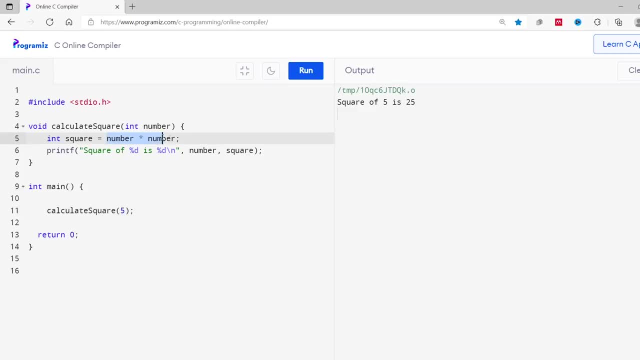 is assigned with the value 5, so when we use number inside the function, we are using the value 5.. a function can also accept multiple parameters. let's see an example here. i'll change this function name from calculate square to add numbers inside the parenthesis. i'll change this number to int number. 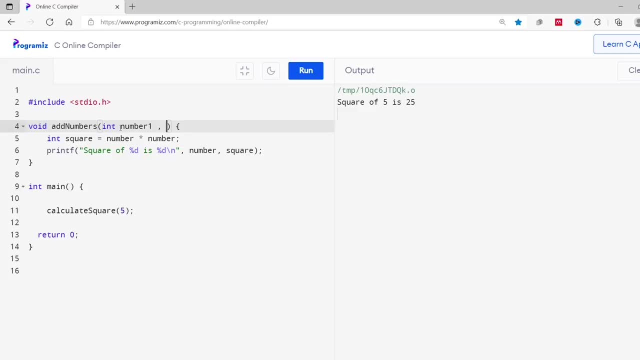 1 and i'll add comma and i'll add int number two. now i'll remove these two lines inside the function and i'll add int. sum is to number 1 plus number 2 and I'll add print statement after that to print the number and sum. so I'll do printf bracket inside quotation: sum of percent d and. 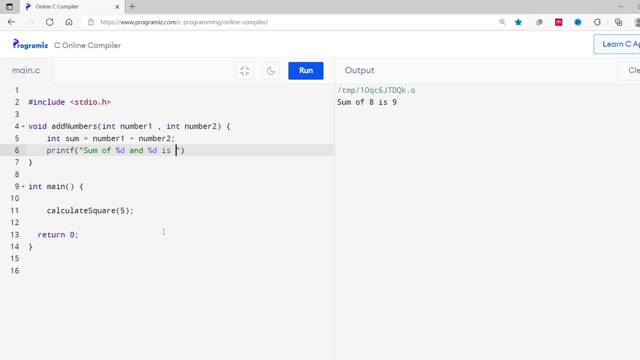 percent d is percent d. that is number 1 comma, number 2 comma sum. now I will remove this earlier function called calculate square and I'll add add numbers with the value 8 and 9 as it's arguments. So I'll run this. As you can see, we get the sum of 8 and 9, that is 17, as output. 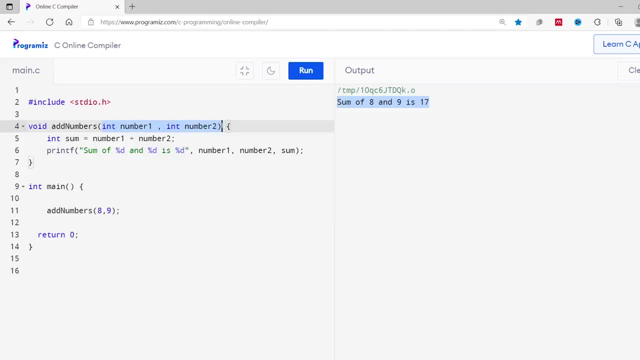 Here the value 8 and 9 are assigned to the parameter number 1 and number 2 respectively. In programming, values passed during the function call are also called function arguments. 8 and 9 in this case are the function arguments. Many people use parameters and arguments interchangeably. 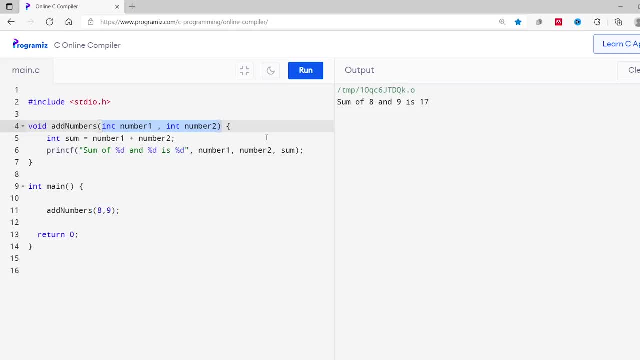 so don't worry about that. However, one thing you should remember is that the data type of parameter and argument should be the same. In our case, we have created in type parameters, so we pass integer values 8 and 9 during the function call If we want our function to accept double or char. 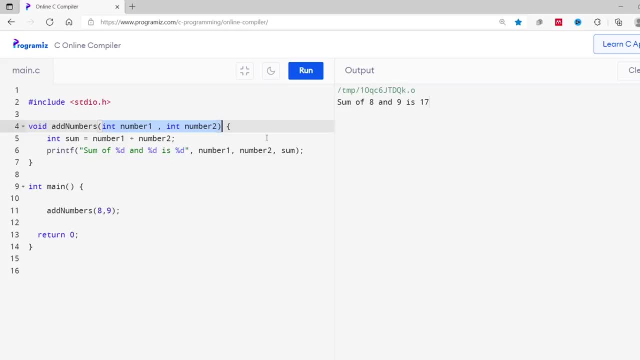 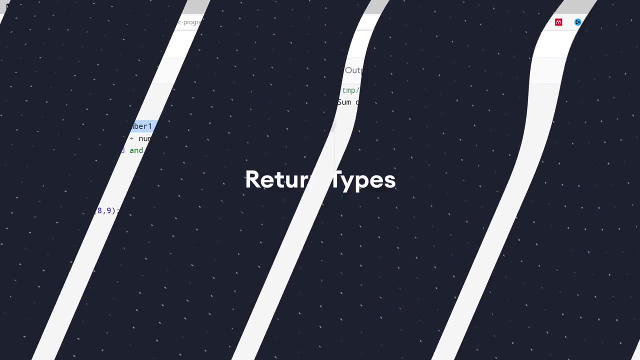 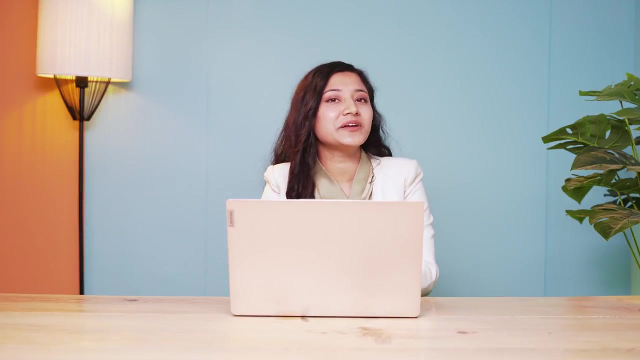 type parameters. we should call the function with double or char values respectively. Go ahead and write a function that accepts double parameters and add them. Till now, we have been using void as the return type of our function. This is because our functions are not returning any value. In C programming we can also create a function that returns a value. 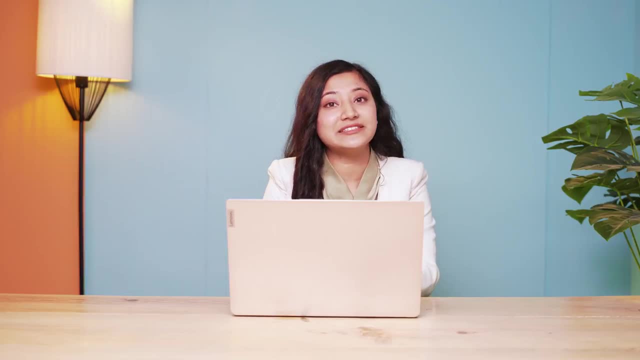 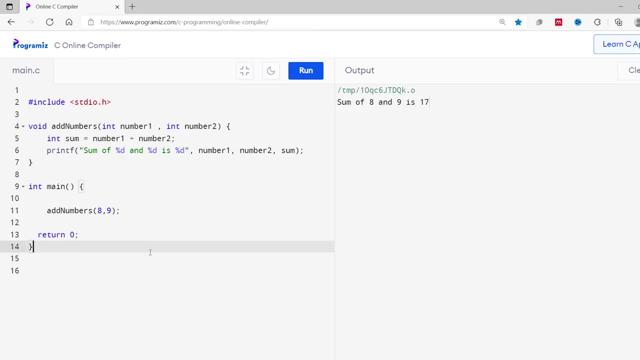 Suppose in our earlier program, instead of printing the sum inside the function, we want to return it. Let's see how we can do that. Here is the code from our earlier program. First, I'll remove this void and I'll add int. I'm using int because I want to return the sum of two numbers and the data type of sum is int. 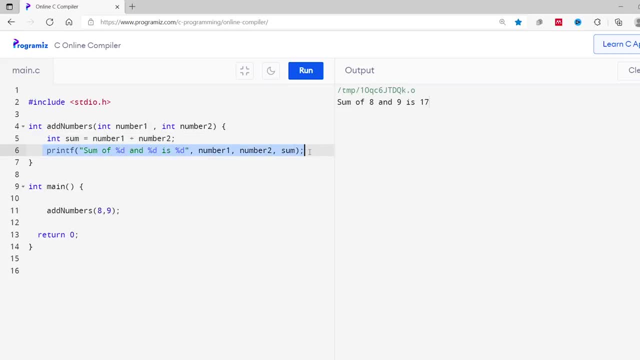 Now I'll remove this print statement and I'll add return sum Here, the return statement that is used to return any value from the function. Since the function is returning some value, this return value need to be stored somewhere. so during the function call I'll assign the function call. 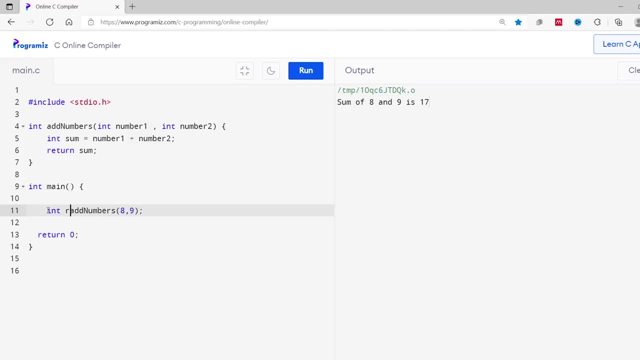 To an end variable, say result. So int result is equals to this function. Then I'll print the result using print statement. So printf result is equals to %d comma result. Now let me run this code. As you can see, we get the result. 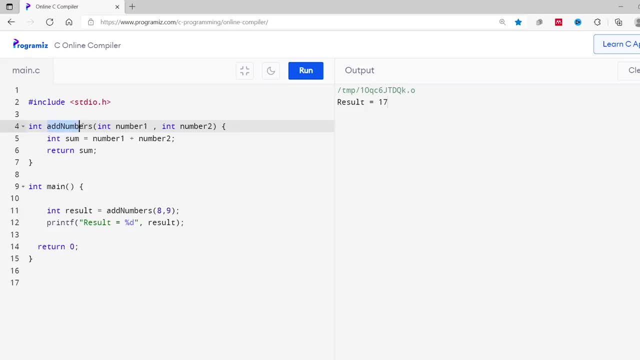 Now let me run this code. As you can see, we get the result. Now let me run this code. As you can see, we get the result Here. the function add numbers add two number, that is, eight and nine, and it returns the sum. the return value now replaces this function. call. 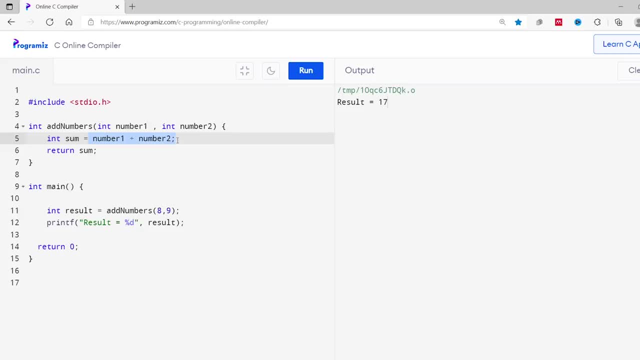 Here the function add numbers, add two number, that is eight and nine, and it returns the sum. the return value now replaces this function call, So this statement becomes int. result is equals to return value, which is 17.. Hence we print the result and we get 17 as our output. 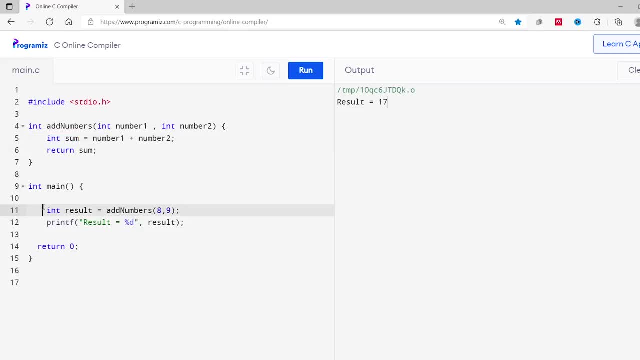 The data type of the return value. we will call the return value and the data type of the variable where the return value is stored should be the same. The return statement is the last statement of a function. when a return statement is encountered, the function exits. We can verify this by adding print statement after the return statement. So 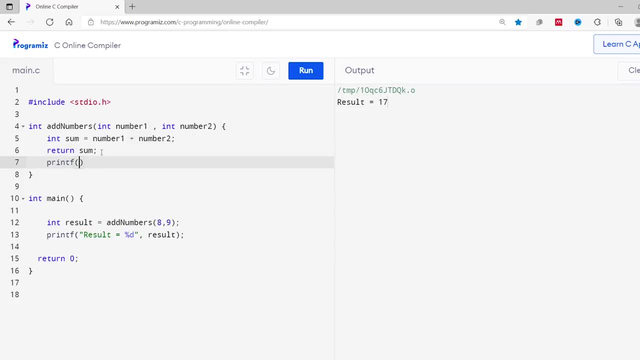 I will add a print statement after the return statement and I will write here after return statement. So I will run this. You can see we get the same output. the print statement after the return statement is not executed. Okay, guys, we need your support to keep these. 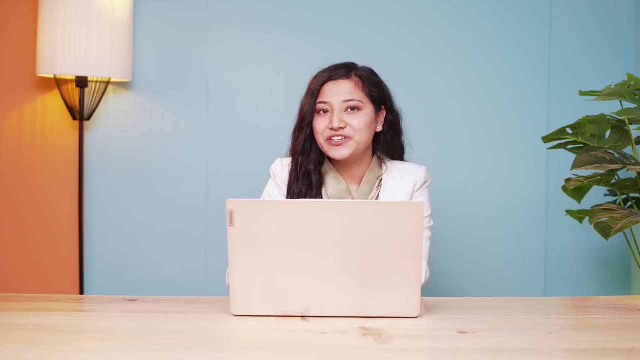 types of content free for all users. YouTube really likes engagement on the video, so leave a comment below, press that like button, hit subscribe if you haven't already. Let's get the engagement score high up so that more people can discover In C programming. a function prototype is a declaration of a function. It provides information. 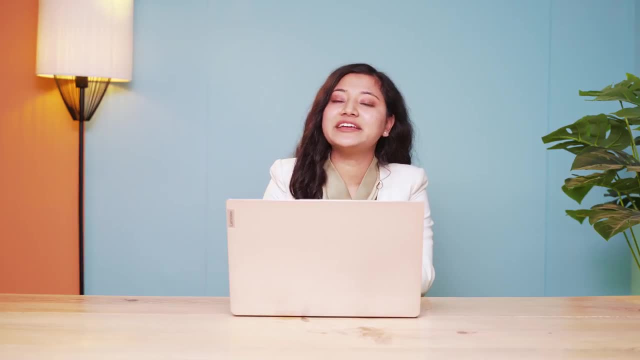 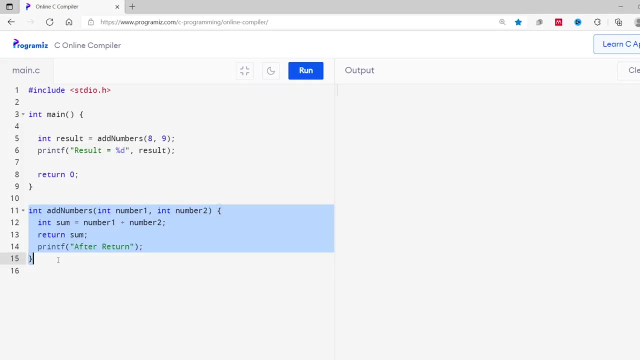 about the function name, parameters and return types. However, it does not include the body. Let's see an example Here. I have the code from our earlier program. If you have noticed, I have put the code of add number function after the main function. Now let me add the function prototype. 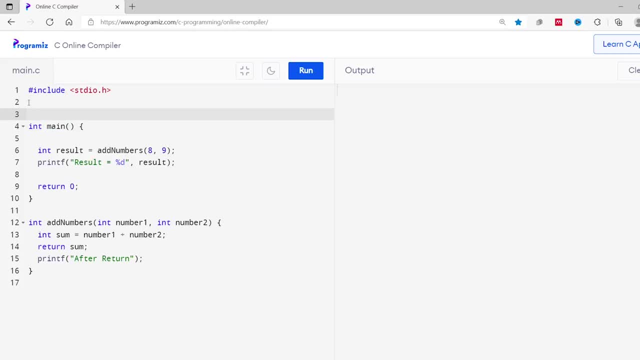 for this add number function, So I will add int- add numbers. parenthesis: int- number 1, comma. int- number 2.. As you can see, the function prototype includes the function name and return type and the parameters inside the parenthesis. Now let me run this code. 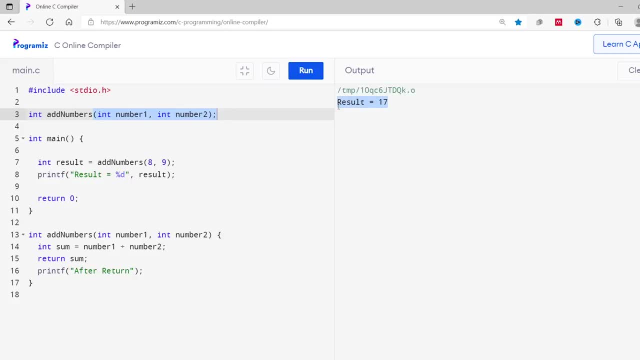 So let's run this code. As you can see, the program runs without any issue. In our program, we are calling the function before defining the function. In this type of situation, the function prototype provides information about the function to the compiler. Now, during the function call, the compiler can now match the function call signature. 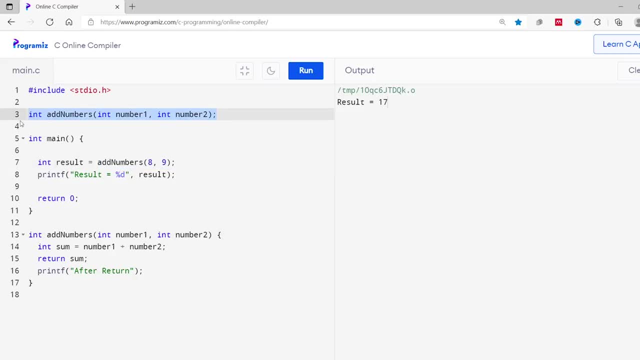 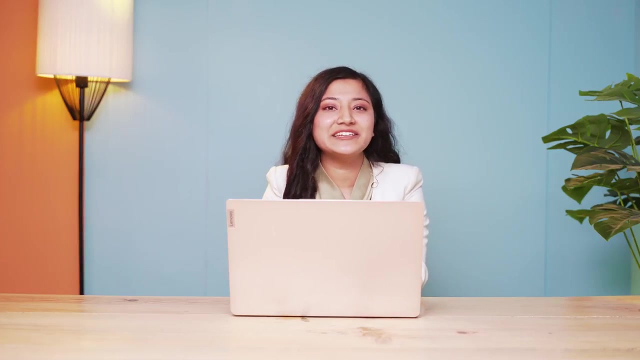 with the function prototype signature If we are defining the function before function call, So the function prototype is not needed. That's why we haven't included any function prototype in our earlier program. So far we have been creating our own function, These types of function. we write the function. 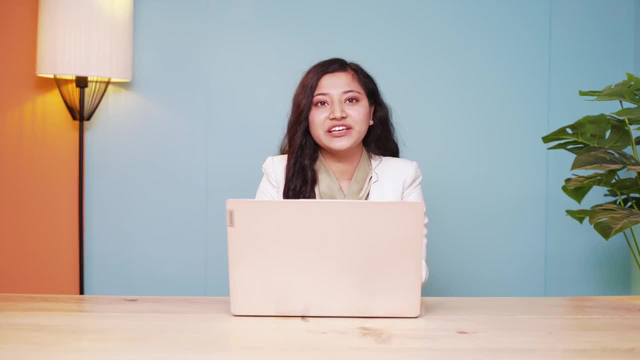 definition ourselves are called user defined function. In C there is another type of function called standard library function. They are built in function that are already defined in the library files and we can directly use them in our program, For example the printf function. The printf function is a standard library function that 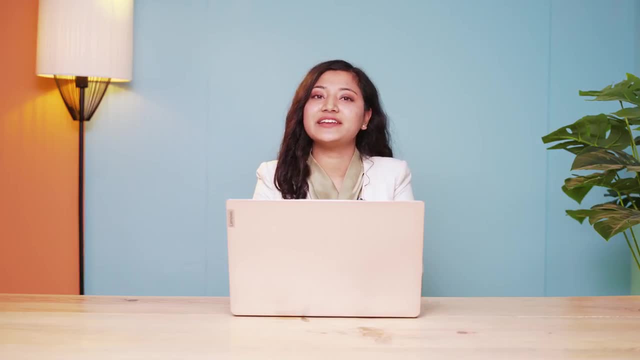 allow us to print the output. The printf function is defined inside the stdioh header file. That's why we need to include the file using include stdioh. Similarly, the sqrt is another standard library function that allow us to compute the square. root of a number. Let me show you an example. Here you can see the basic C program. First we need to include math header file, because sqrt is defined inside the math header file. So I will include math header file. 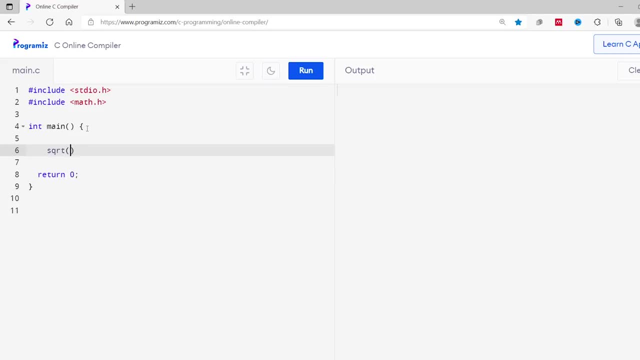 Now, inside main, I will use sqrt function. The sqrt function returns the square root of number as a floating point value, So I will write float result. So I will write float result. So I will write float result. Sqrt is equal to sqrt and inside sqrt I will write 25 and I will end this with semi colon. 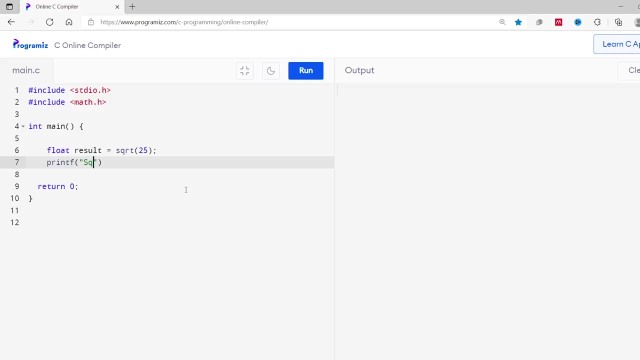 Now I will print this square root. square root is %f, comma result. Now I will run this code. As you can see, we get 5 as output, which is square root of number. So it is a good, but I am not going to print it.